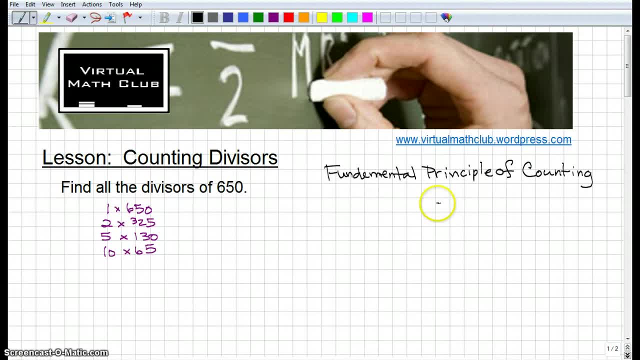 principle. obviously It's called the fundamental principle of counting Um. you might know it as the product rule, And what it says is is pretty basic. It basically says: if you have, let's say, n ways of doing one thing and m ways of doing another thing, then you can just multiply n times n, m times n or n times m um to get the number of ways to do the combination of the two things. Okay. So, for example, let's say: 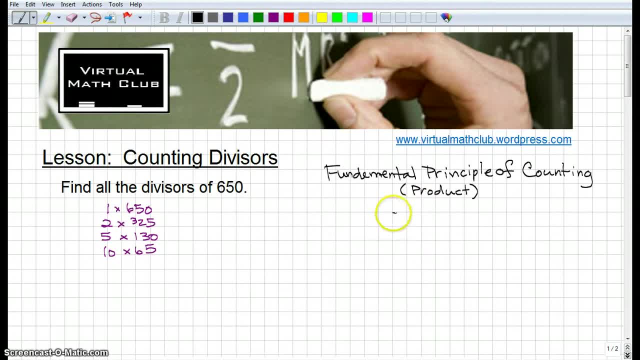 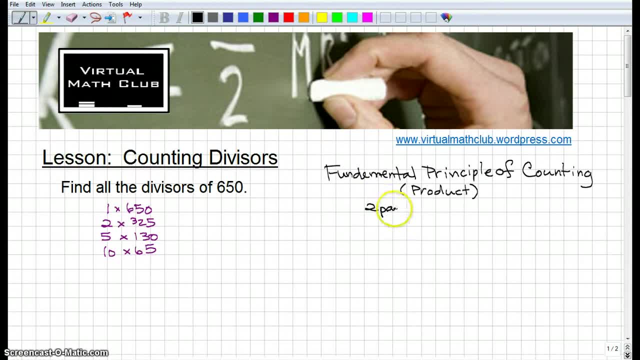 let's say I have two pair of pants and let's say I have three shirts, then if I want to know how many outfits I can create- this- I mean, all these pants are different and all these shirts are different- if I want to know how many outfits I can make, I can just take two times three, because I have two choices. 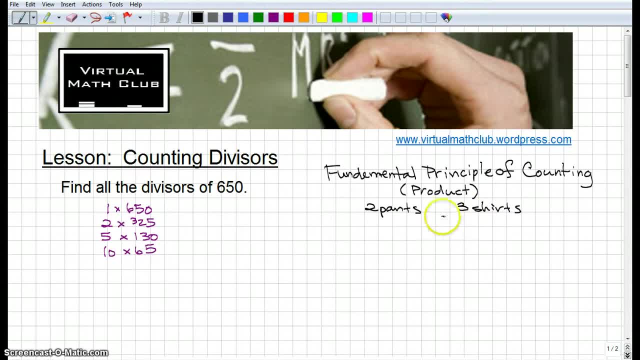 for pants and three choices for shirt, and once I have a pair of pants and a shirt, I've got an outfit. basically so, and you can see that in the tree. if, if I show my two options, maybe I have jeans- oops, jeans, and let's say I have khakis. 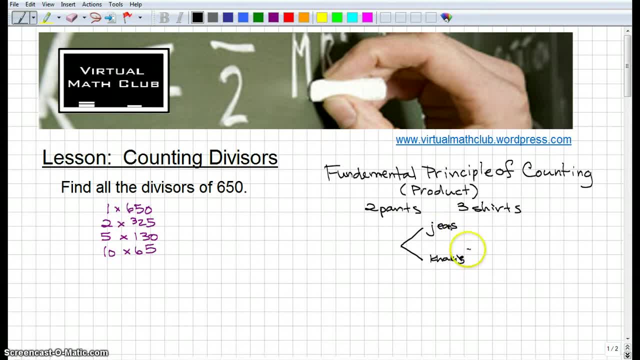 khakis. all right, those are my two choices for pants, and maybe I have a red shirt and let's say I have a yellow shirt and let's say I have a blue shirt. okay, so if I choose the jeans, I have three choices for shirt and if I choose the 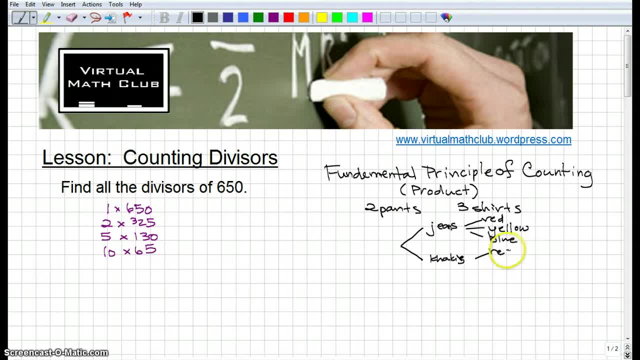 khakis, I have the same three choices of shirt. okay, I don't have anything clashing, so the so the choice of shirt is not dependent on my choice of pants. okay, maybe if I had a pair of purple pants, maybe I wouldn't want to wear them. 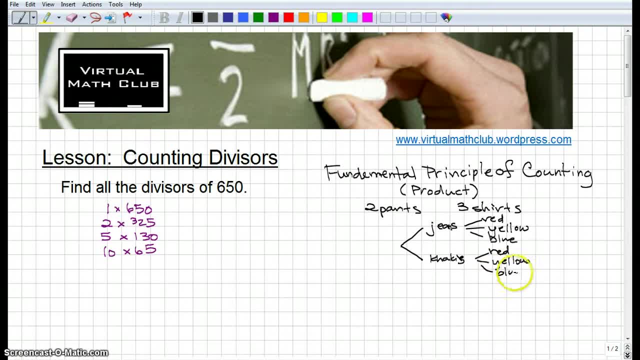 with a red shirt, I don't know, depends on what your taste is. okay, so you can see how we we get. I don't know, I don't want to wear them with a red shirt, I don't know. 75%. so transportation is the most important thing today. I think those are a lot of. 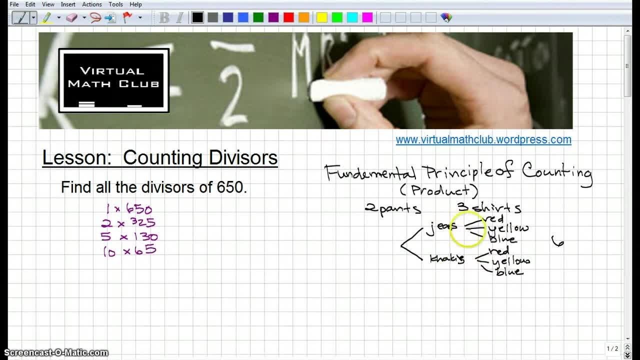 the options for sickness, for eligibility, and I that I absolutely recommend that that search what we get. I love getting six outfits and these basically show you all the possible outfit. we get this of jeans with the red shirt, jeans with the yellow, jeans with blue or the khakis with the Red, Hatchies with the Gallow, khakis with the Blue. 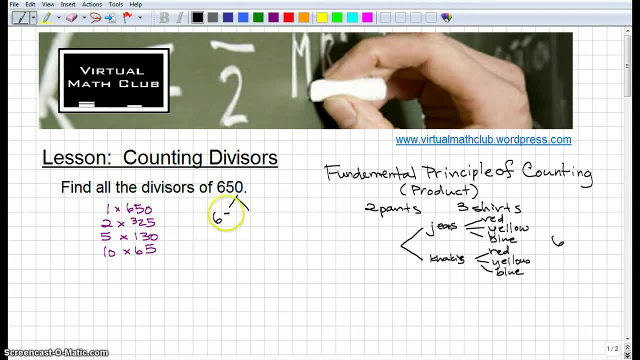 alright, so let's go back to this, finding the number of divisors of 650 and it, we can factor this into 65 times 10, and we can factor 65 into 5 times 13. right, and 10 factors into 2 times 5. all right, and now all of these numbers, here are: 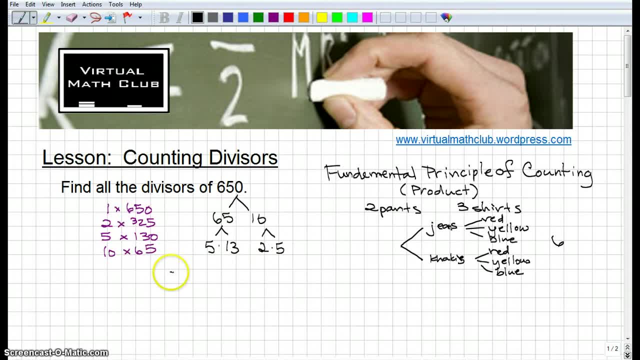 prime, so the prime factors of 650. if I write 650 in terms of its prime factors, I get 2 times 5, squared times times 13. okay, so those are the prime factors, and all of the factors of 650 are some combination of the prime factors of 650. 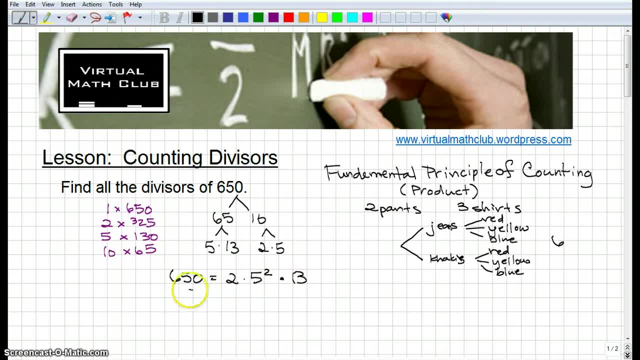 okay, so the, so the. the factors of 650 have are made up of these prime factors. okay, 13 is obviously a factor. It's also a prime factor. I can take 2 times 1 of the 5s, and that's a factor. I can take 5 times 13, and that's going to be a factor I can. 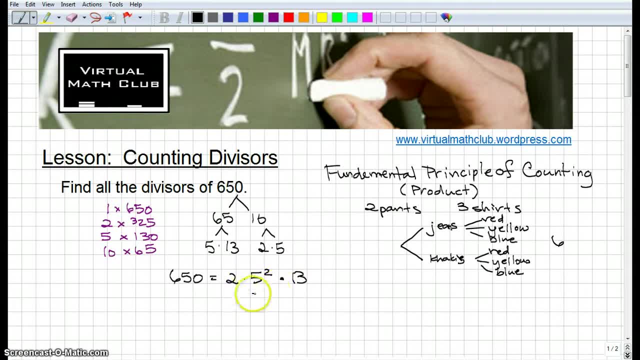 take 2 times 13.. That's going to be a factor, So I can create different combinations of these prime factors and that will give me all the factors of 650.. So the question is: how many ways can I put together these prime factors in order to get all of these divisors? I guess I'm using divisor and 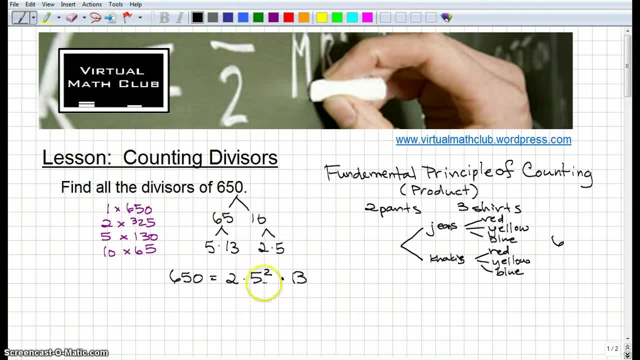 factor interchangeably, but these are the prime factors. So how can I use these prime factors to create combinations that give me all the divisors of 650? All right, so here's the trick: A divisor of 650 can actually be a divisor of 650. 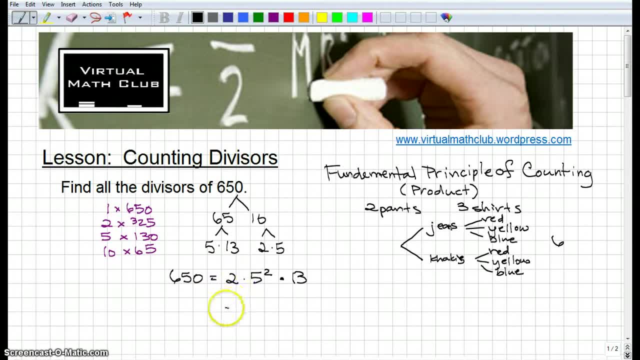 a divisor of 650 can actually be a divisor of 650.. We can either have no 2s, 0 2s, or it can have. I'll write the options down here. We can have 0- 2s. 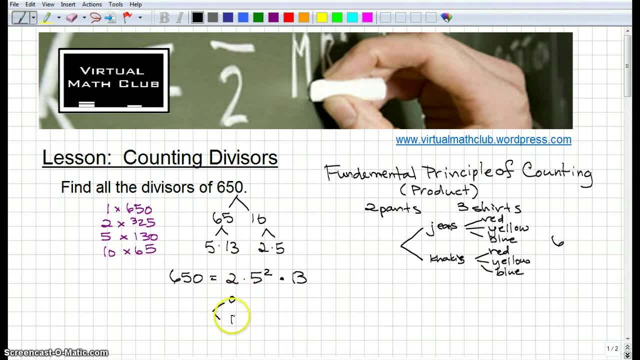 or we can have 1, 2.. Okay, those are our choices for the power of 2.. So 2 to the 0 is just 1.. That just means that it doesn't have any factor of 2, okay. And if it has 1, 2, that's. so 2 to the 0 is. 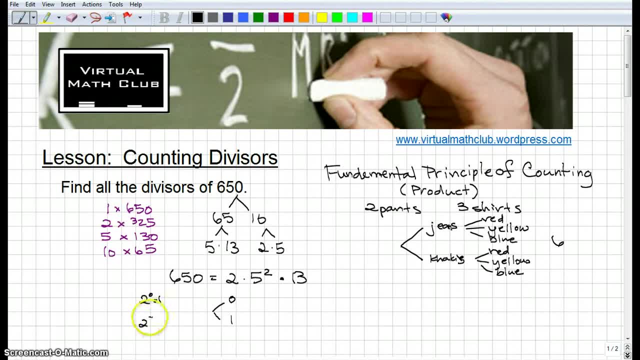 1. So that means we have no 2s And 2 to the 1 is 2.. That just means we have 1, 2, okay, And our choices for the factors of 5, we can have no 5s, We can have 1 5s or we can have 2 5s. 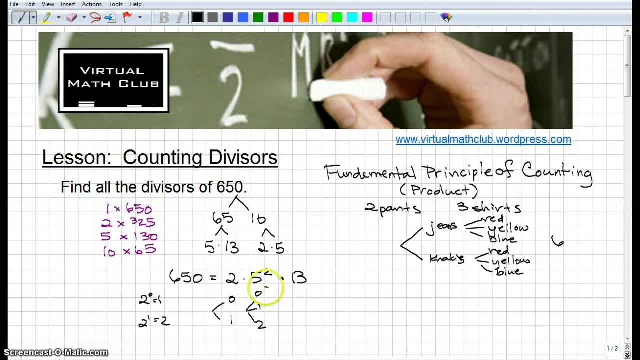 Okay, so we have actually 3 choices for the, for how many 5s are in our divisor, And then for 13,. that's just, we can either have 0,, we can have no 13's, or we can have 1- 13.. Okay, So basically we have: 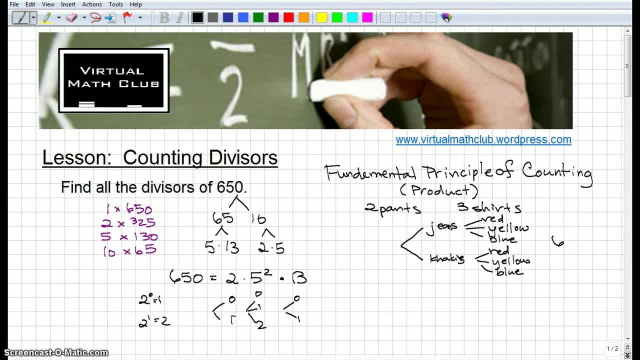 two choices for how many twos to include in the divisor, We have three choices for how many fives to include in the divisor, And we have two choices for the number of thirteens to include in the divisor. Okay, and if we come up with all those combinations, we'll get it. So you can see, we 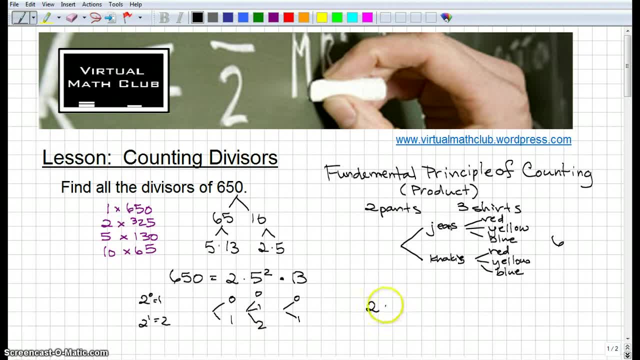 have two choices for the number of twos. We have three choices for the number of fives and two choices for the number of thirteens, which should give us 12 divisors of 650.. So obviously I only have eight. so there's a couple missing right, And let's take a look at what the tree would look. 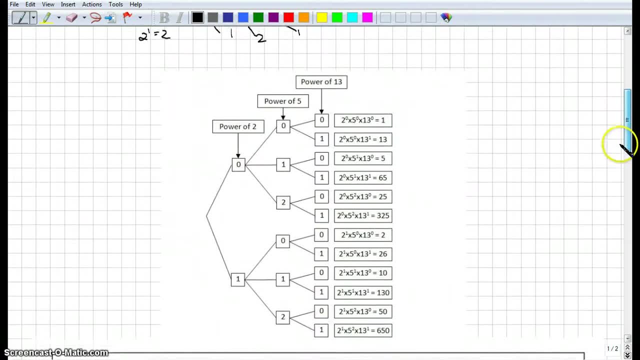 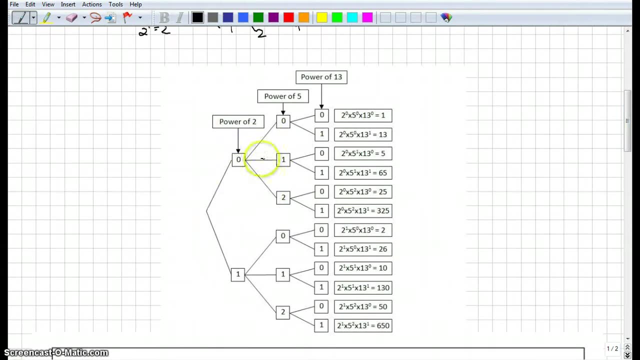 like for all the different options of 600, for the power, for the, for all the different divisors of 650.. Okay, so basically, here's our, our, our choices. we have, we have a factor of two. we can either have one, one, two or no twos, do you? 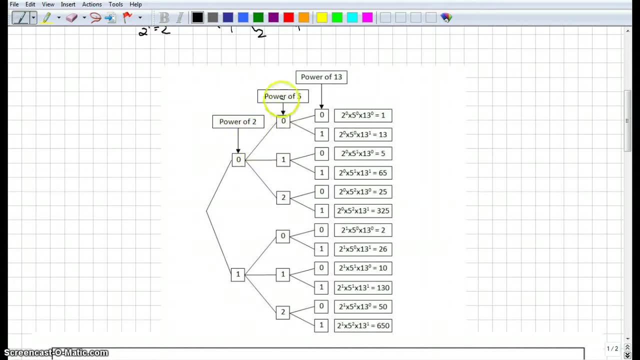 see And fat the power of five. we can have no fives, we're gonna have one five, or we can have two fives, one then, and we independent, you know, and independent of how many, how many factors of. 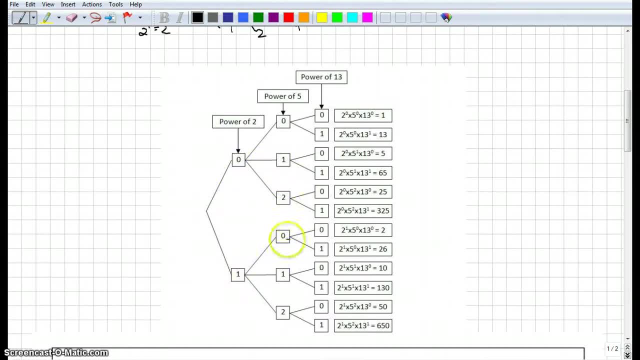 two, we still have three choices for the power of five. okay, that just tells us how many fives are we including in that divisor? okay. And then again we have two choices for the number of thirteens to include in the divisor. And here are all the factors. if you multiply that out, 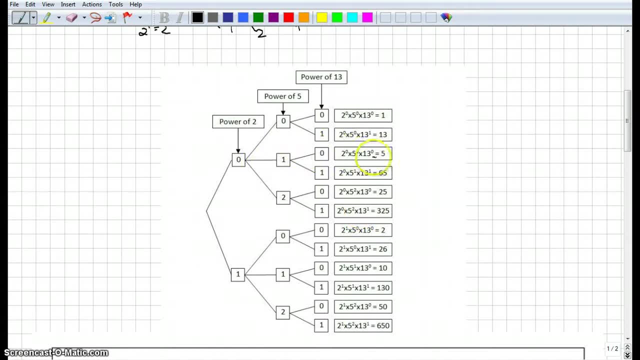 If you trace through any branch of the tree, you'll get a unique divisor of 650.. Okay, so, for example, this branch- let me use a highlighter- this branch. this tells us we have highlighter, we have no twos. 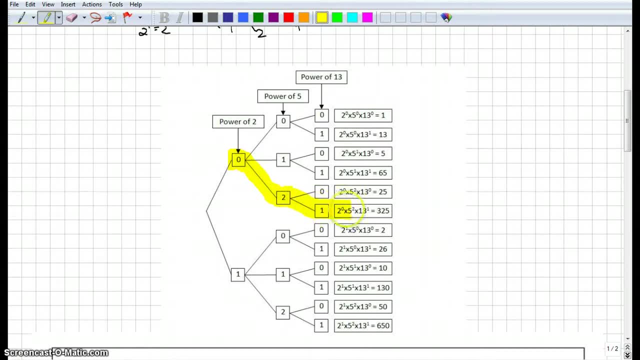 We have two fives and we have one thirteen, which gives us 325, which is one of the divisors of 650.. If we look at another case, here we have one, two, we have no fives and we have one thirteen which gives us the 26.. 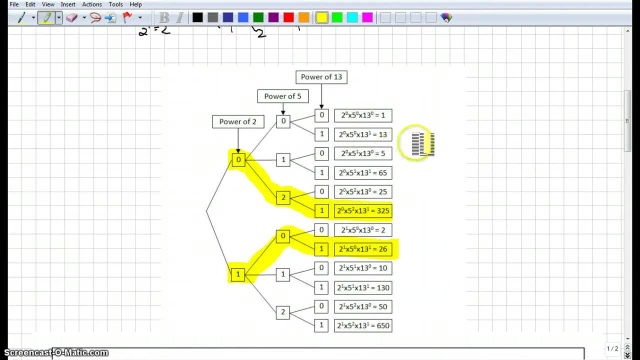 Okay, so each one of those branches on the tree is going to give us a unique divisor of 650.. Alright, so the general rule for any number. if we want to know how many factors it has, we just need to. we need to, first of all. here's the steps. let me write them out. 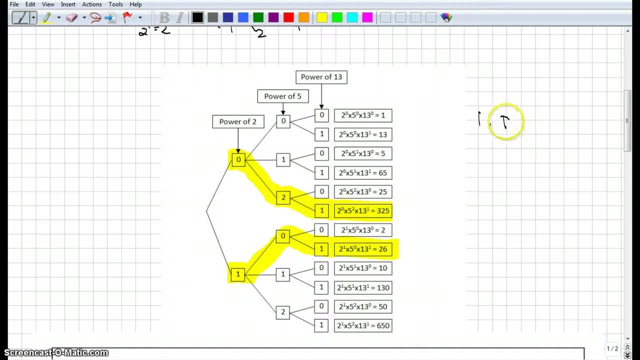 So the first step is to write the prime factorization. Okay, so we look at the prime factorization and then we look at the exponent of each prime factor. Exponent of each prime factor- And we have to account for the fact that zero is an option. 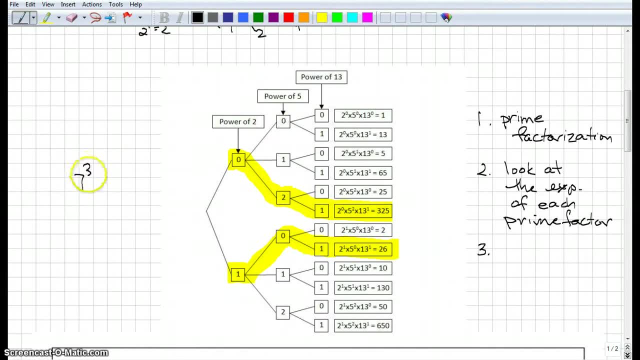 So if we have, say, seven cubed in our prime factorization, then we can have zero sevens, we can have one or two or three sevens. so that gives us four options. So we need to add one to each. so let's see, add one to each. 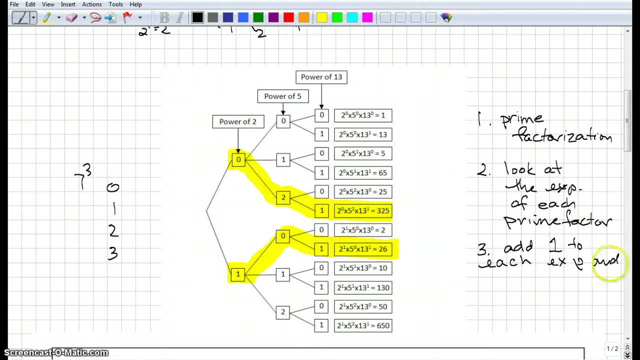 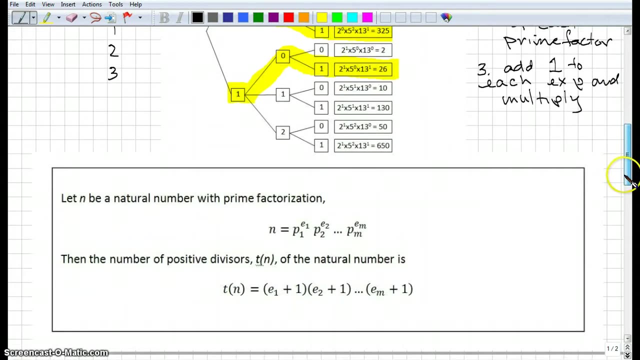 comment: exponent, exponent and multiply And that will give us the number of factors divisors that that number has. So here is the rule written in mathematical notation. So if we have N and we write it in terms of its prime factors, 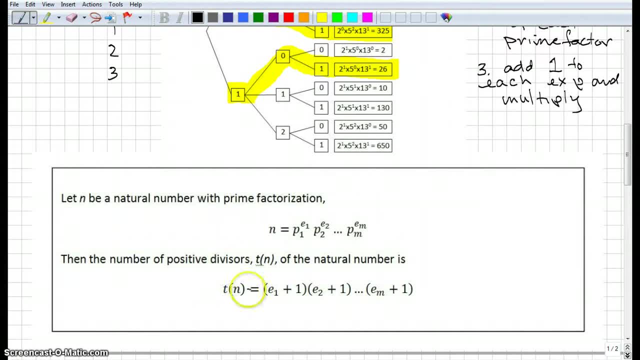 Then the number of positive divisors that that prime number has is essentially the exponent plus one times the exponent, the next exponent plus one times the next exponent plus one. so you just take all the input exponents, add one and multiply. okay, so let's do another example: all. 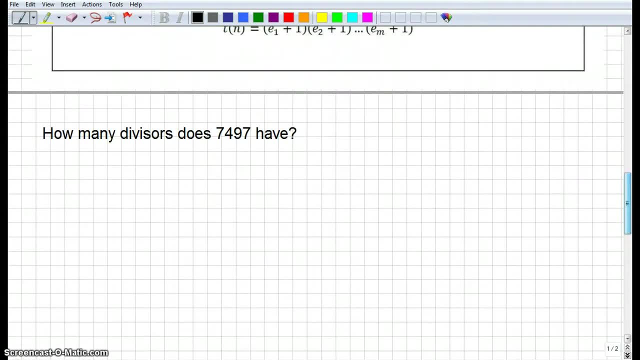 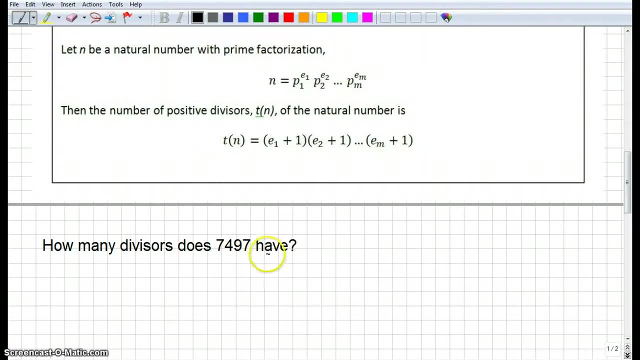 right, let's look at this one. this is a lot harder. we want to find all the divisors of- well, we can leave this up here just so for reference- of seven thousand four hundred and ninety seven, yeesh, okay. well, the hardest part of this one is just finding the factors, the prime factors. so I know it's not. 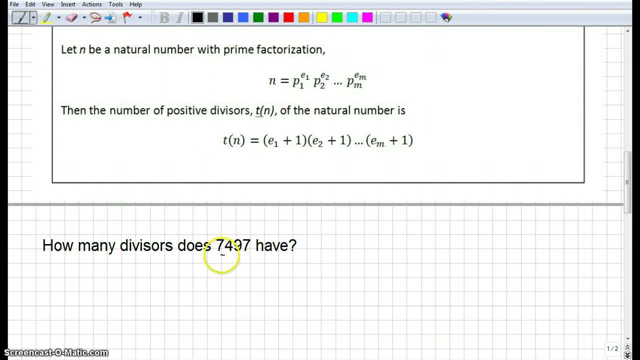 divisible by two, because it's not even. let's check three. I have 11 and 16, which gives us 27, that's the digit sum, and 27 is divisible by two, because it's not even. let's check three. I have 11 and 16, which gives us 27, that's the digit sum, and 27 is divisible by. 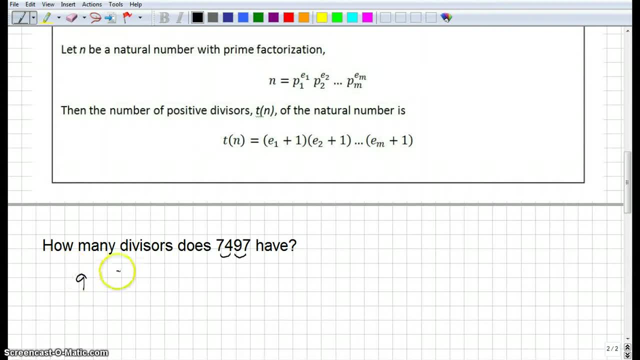 three, but it's also divisible by nine. so I know this number is divisible by nine, so I can actually take care of two, threes by dividing this number by nine. okay, so what do we get when it's the when we divide by nine? well, we get. let's. 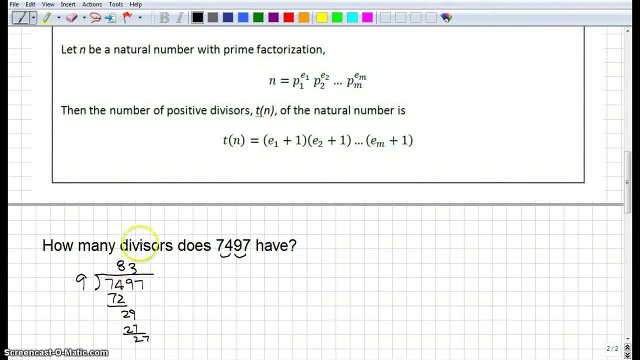 see, that's three, twenty seven, twenty seven. that gives us 833, okay. so the first two factors are nine and 833 okay. and then this is three times three. so there we have that part of it down into prime factors. now let's look at 833. that's not. 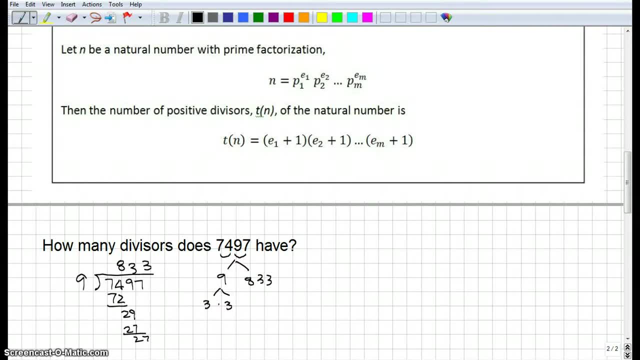 an easy one either. it's not divisible by two, it's not divisible by three because the digit sum is 14 and that's not going to work. it doesn't end in a zero or five, so it's not divisible by five. so let's try seven. let's just try this out. 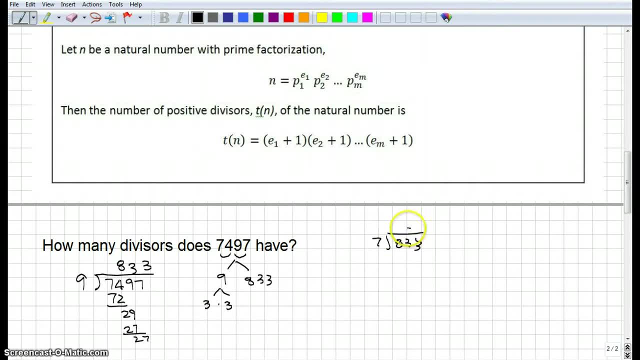 833. if we divide it by seven, we get, let's see, one, seven, thirteen, let's see. I guess I just couldn't do a one seven. and then I'm left with what: 63 and nine. oh, so good. it's divisible by seven and it's seven times 119. all right, well, now we. 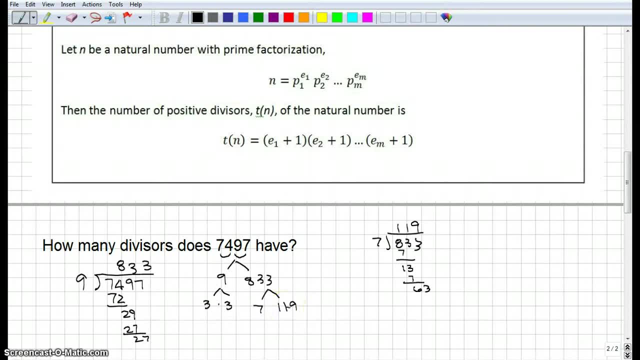 know 119 is divisible by seven and it's seven times 119. all right, well now we know 119 is not divisible by two or three or four or five again, because this 833 was not divisible by any of those numbers. so let's try seven again. all right, seven. 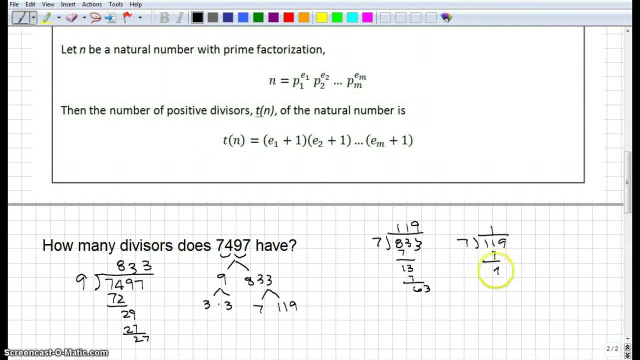 one, one, nine, let's see seven. that gives us 49. oh, look at that, hey. so this is seven, seven times 17, all right, and we know 17 is prime. so our prime, factorization is, factorization is and again, like I said, this is the hard. 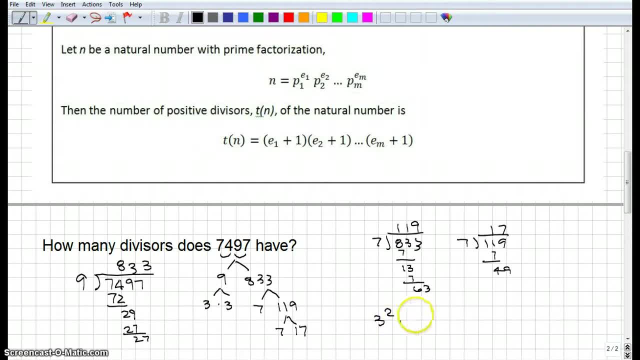 and again, like I said, this is the hard part: 3 squared times 7 squared times 17. part 3 squared times 7 squared times 17. so how many factors do we have 7497 we? so how many factors do we have 7497? we have 3 times 3 times 2 is well, it's 18. 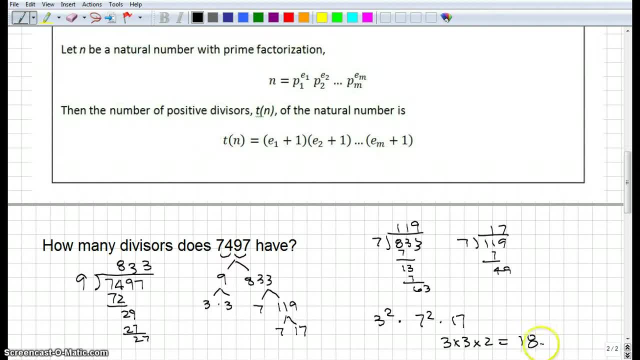 have 3 times 3 times 2 is well, it's 18, right? so we have 18 factors of, or we, You could say divisors of, 7,497..